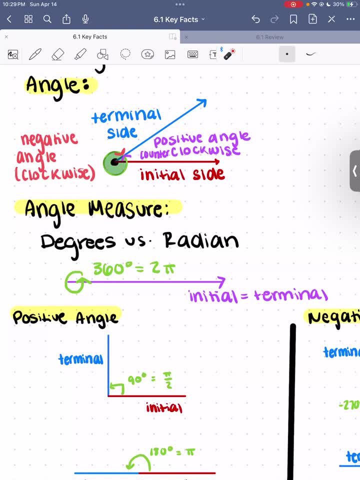 Okay, so what do we measure angles in? So we measure angles in either degrees or radians. So I'm sure you guys have heard of both, whether you think you have or not, But typically how we define our big angles here. So for degrees, I'm sure you've heard of 360 degrees. 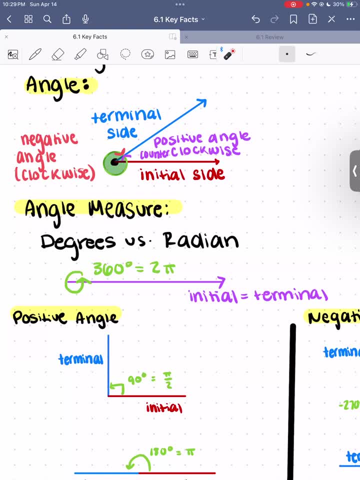 180 degrees, 90 degrees, very common, And you know that's usually signified by this little circle degree mark right here. And for radians, I'm sure you've heard of pi, which is 3.14. But for radians we kind of just like to use our symbol, pi, instead of. 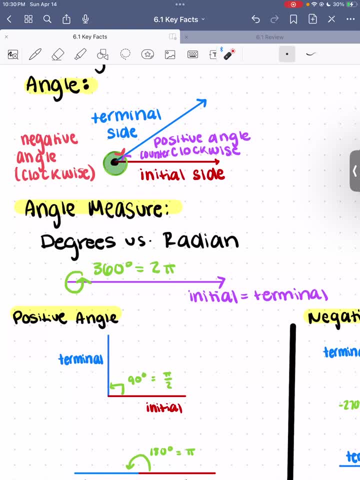 actually saying 3.14.. So if the initial and terminal side are the same, so that means that can be shown on this just purple line. So that means they are exactly on the same line. So if you measure that one complete from this side going to the other side. 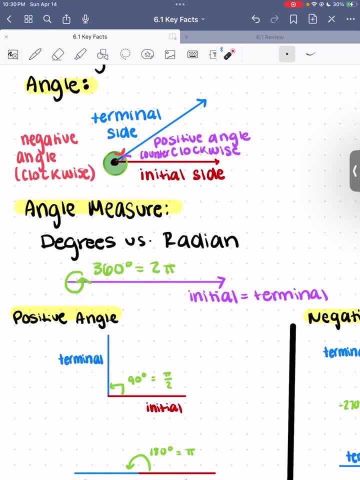 the measure of 360 degrees or two pi radians. So if you want a visual, if you think of a circle, if you start at a point on a circle, go entirely around so you reach that same exact point. you would have gone around 360 degrees or you would have gone around two pi radians. 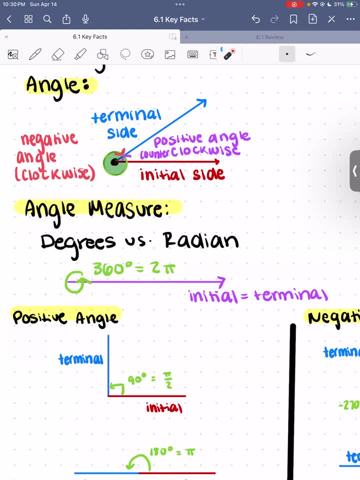 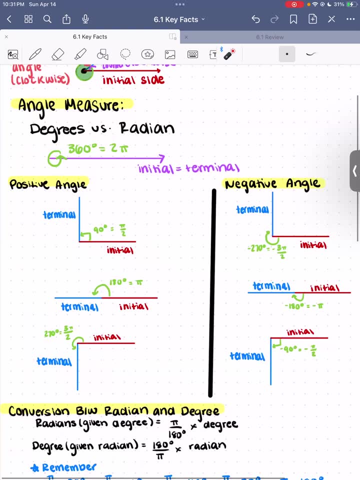 They equal the same thing, It's just a different way of showing it All right, Now that we know that, and since we've already talked about positive angles versus negative angles, let's show some very common angles in both degrees and radians. So, starting with, we'll start with the positive. 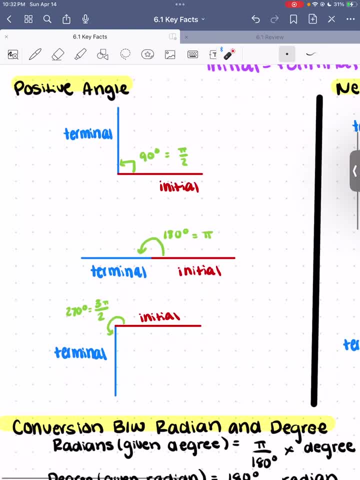 angles on our left here, Whoops. Okay, So here we have our initial side right here. If we go and do this and, as you can tell, it kind of looks like a box, If we were to complete these other sides it would be a square, And if we go from a flat, 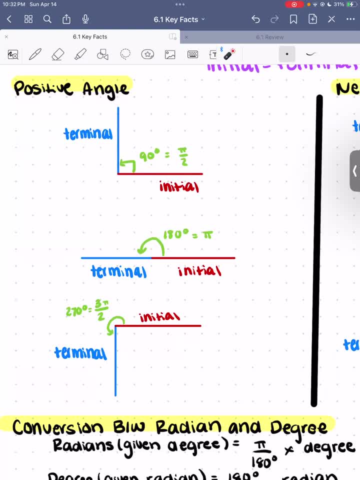 so our flat initial point to a terminal side which is completely vertical, straight, a straight vertical line. we have gone 90 degrees or we have gone pi over two radians. They mean the same thing. So remember, if we've gone 90 degrees or pi over two radians, it's when the terminal side 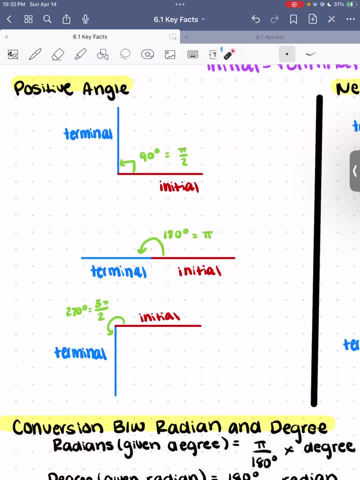 is a straight vertical line And that is a vertical line upwards for a positive angle. So if we go and do this and as you can tell, it's a square, And if we go and do this and, as you can tell, it's a straight vertical line upwards for a positive angle, So going this way, Remember. 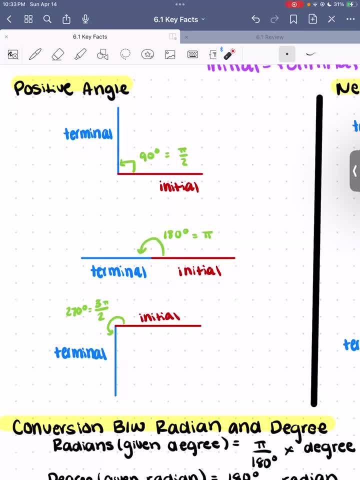 counterclockwise. so, if you think about it, here we go. we've gone 90 degrees counterclockwise, or pi over two radians. Okay, we're on to our next one. So here we have our initial side and we also have our terminal side. As you can see, it is completely, it's a straight. 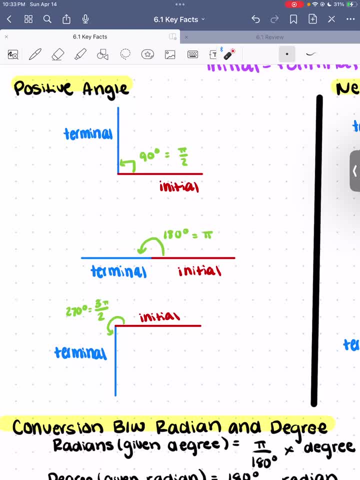 line. This is a vertical line, Remember. we always have to start from our initial, though, And since we're talking about positive angles, if we go counterclockwise, just this way, we have gone 180 degrees, or pi radians. So 180 degrees, or pi, is a straight vertical line from one another, going measuring. 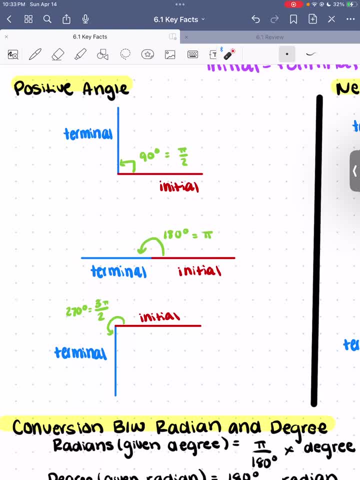 in our counterclockwise direction. So that's important to remember. And so now here's kind of something that I wanted to differentiate between: 90 degrees and pi over two is our 270 degrees and three pi over two, So three pi over two radians. So 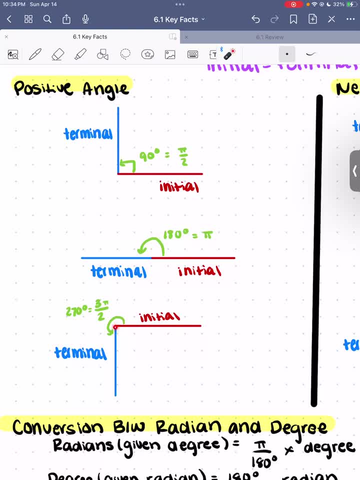 if we have our initial right here, once again, we have another terminal, vertical terminal side. However, this is not 90 degrees because this is facing downwards, So we do need to travel a little bit farther. Remember, we always want to start from our initial go. 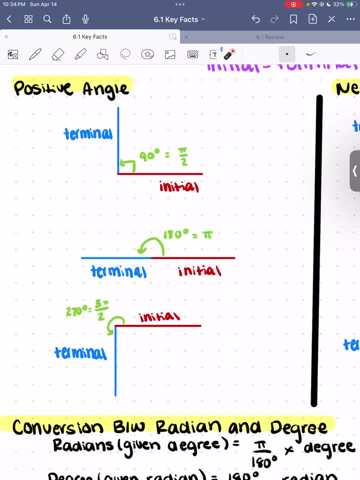 to our terminal side. So, but since this is in the case for a positive angle, so we have to travel counterclockwise, So we have to travel a little bit farther, And that's how we get 270 degrees or three. 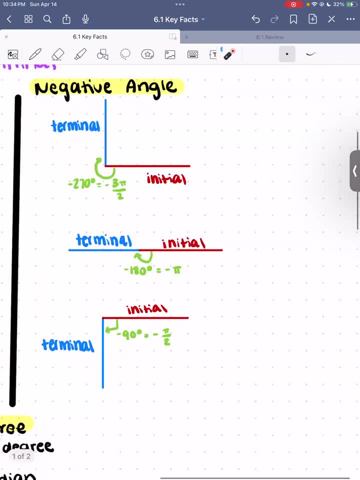 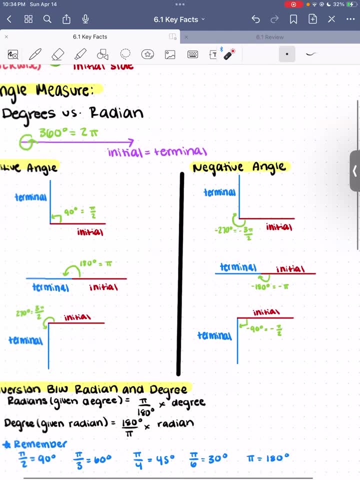 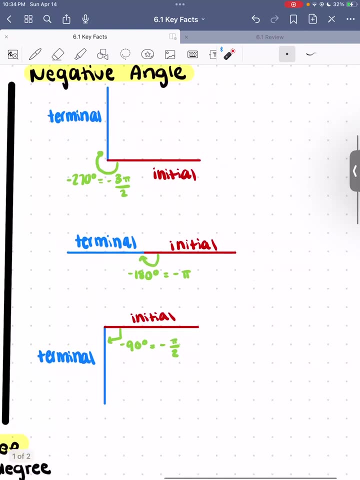 pi over two radians. Now let's say we were measuring it negatively. So now you can kind of see just by comparing both we kind of have the opposite thing going on here. But let's start. Okay, I'm actually going to start at the bottom here, since we started with 90 last time. 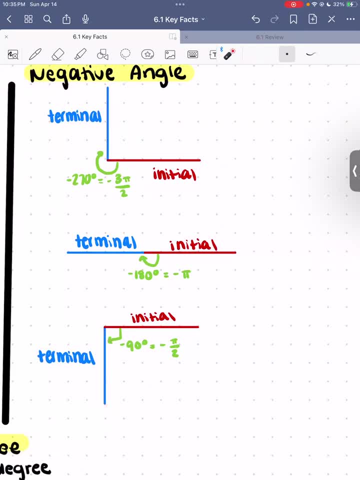 So we have our initial and we have our terminal, And we just discussed a similar problem, but in positive. However, since we're going measuring the negative angle, we still start our initial, but instead we're going to move clockwise. We're going to move clockwise to our terminal. 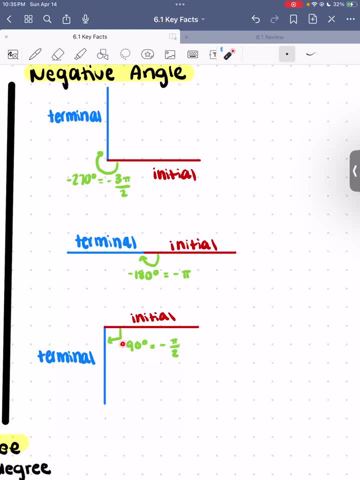 angle or our terminal side. So when we do that, remember our angles and our radians need to be negative. So we have just gone negative 90 degrees or negative pi over two radians. So when we're comparing our initial and terminal here in this example, it does look pretty similar. 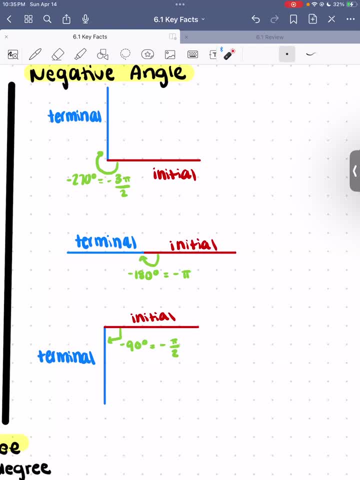 to our 180 degrees or pi, because still it is still a straight line. However, if we measure clockwise instead of counterclockwise, it's still going to be 180 degrees. Remember, measuring clockwise gets us our negative angles, So it'll just be negative: 180 degrees or negative. 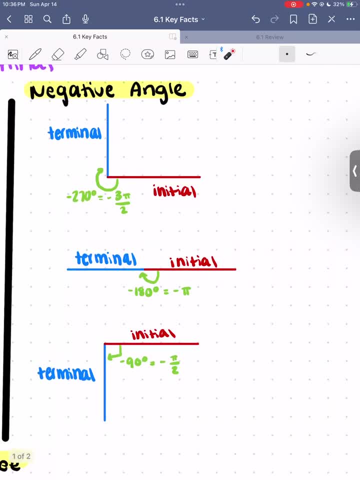 pi. Now to our top example. looks like our 90 degree one, with our initial here and our terminal being a vertical line here. But instead of measuring counterclockwise, we're measuring clockwise. So since we have to move a little bit farther, we're not doing 90. We have a 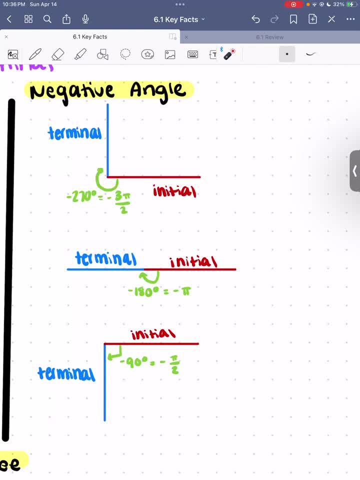 closer to a circle. You can kind of see that. So we're just going to go counterclockwise, Okay. So this would be our 180 degree one And what you can see, that when we come back from the excess, we're actually going to be able to get this in temperatures. But it's actually 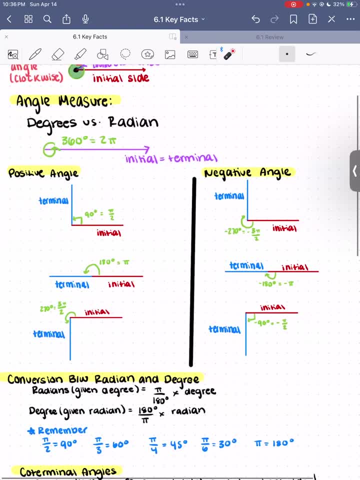 going to be a little up. So if we see which one of these this is- negative 180 degrees or negative three pi over two radians, We're going to have negative one over two radians. If you are able to see the comparison here, you can see like comparing it right here. 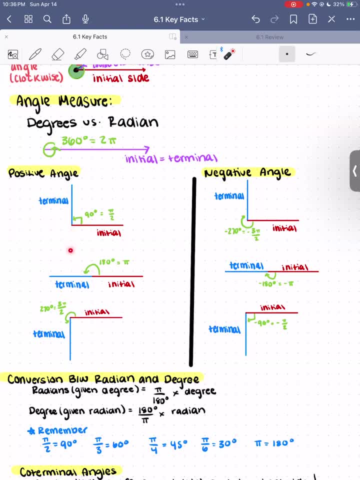 This would be where our 180 degrees would be, And here is where our 180 and here's where our 270 would be. If you can tell the difference, they're all 90 degrees apart. So they're all 90 degrees apart. 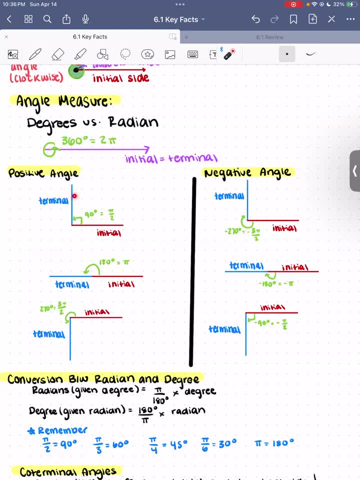 part. So if you can't remember, just know that the first one is 90, the next one is 90 more, which is 90 plus 90 is 180.. And if you go down to our next down vertical, it's. 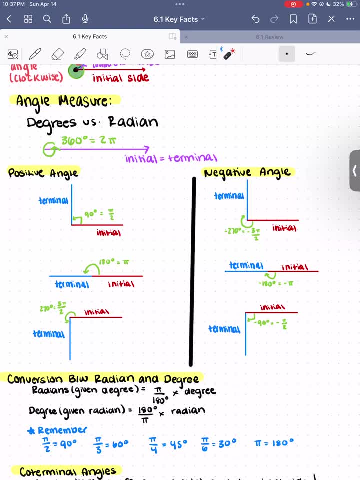 180 plus 90,, which is 270.. Same thing with our radians, except that they're all pi over 2, apart This one's pi over 2,. this one is pi over 2 plus pi over 2,, which is pi Then. 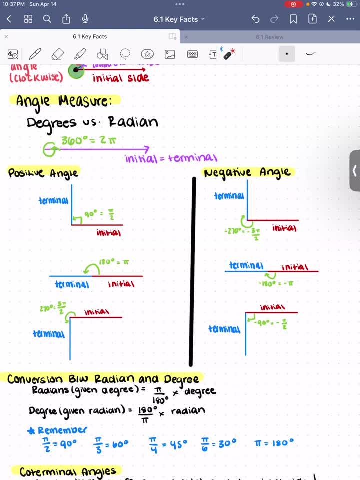 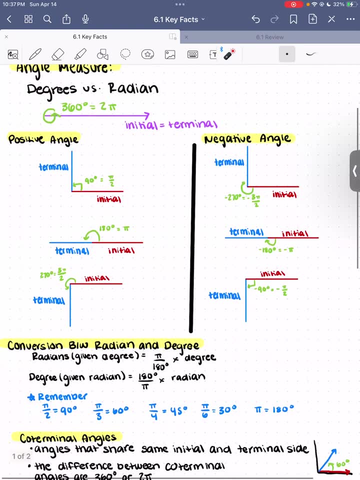 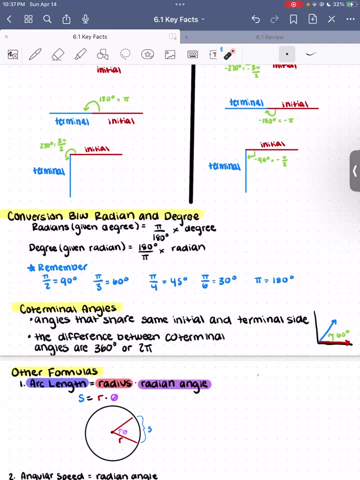 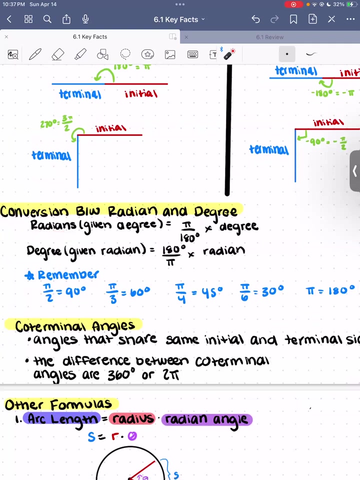 if we go down again, it's pi plus pi over 2, which is how we get 3 pi over 2.. Okay, so now we talked a lot about radians and degrees and what they're equal to each other, but how do we do these conversions? So, whenever you want to go from radians to degree mode, 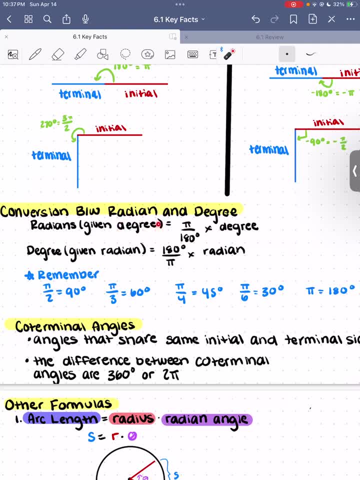 or to degrees. that means you've been given a degree And you want to get to radians, And so the equation for that now you need to remember, is pi over 180 times the degree you just got. The way I remember this is is if our degree 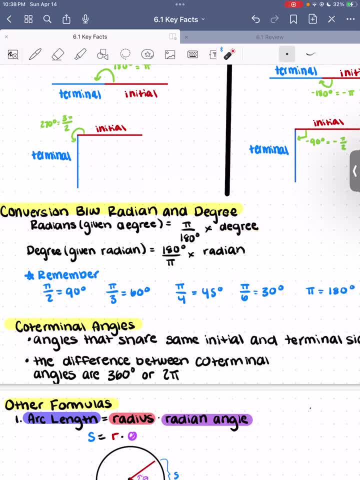 is right here. remember, when something's in the numerator and something else is in the denominator that are equal of the same unit, that unit's going to cancel out. So since we want to get into radians, which is usually shown in terms of pi, we're going to want our pi on top. 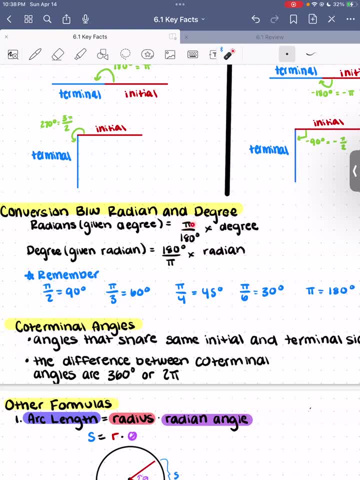 So that's how we know we want to get radians, because we want our pi to be in our final answer. And just remember how do I like pi over 180, remember that pi and 180 are equal to each other, So that's why they're both used here. Now, oppositely, if you're given 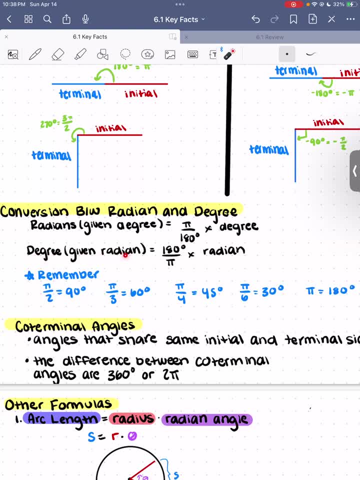 a degree, or you want to get a degree and you're given a radian. it's going to be the same formula, but just flipped, except we have 180 on the top because we want our answer to be in degrees. so we want the degree to be on top and we want pi to be on the bottom. 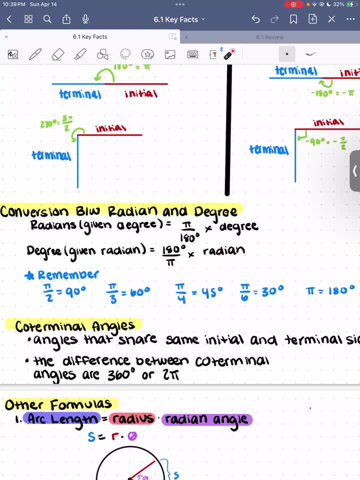 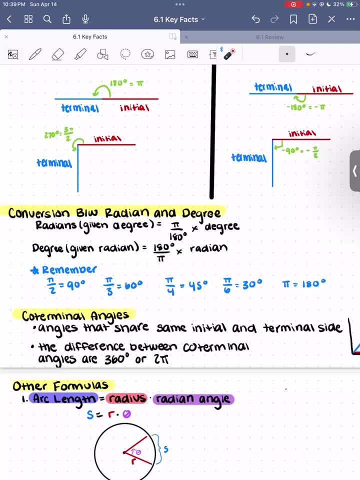 because it'll cancel out with our radian over here. So- and I'll do some examples later in another video that you can check out- but just for some key things to remember or that you should be able to remember, or I would offer remembering these because these will. 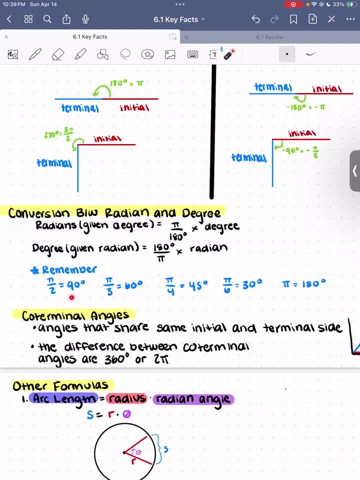 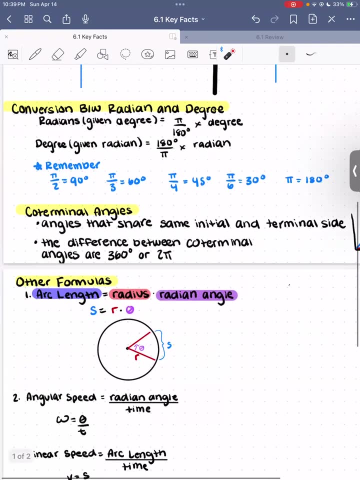 come up a lot throughout trig. So pi over 2 is equal to 90,, pi over 3 is equal to 60,, pi over 4 is equal to 45, pi over 6 is equal to 30, and pi is equal to 180.. Okay, so let's. 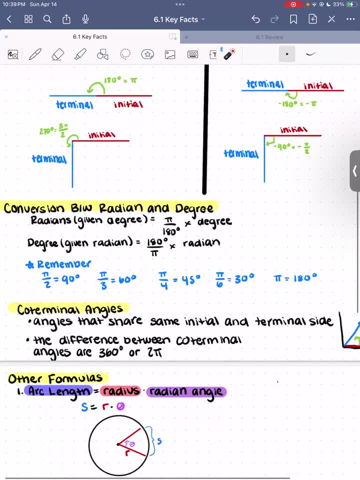 talk about coterminal angles. Okay, so, let's talk about coterminal angles. So let's talk about coterminal angles. Okay so, let's talk about coterminal angles real quick, before we go too far. So what is a coterminal angle? So, a coterminal angle. 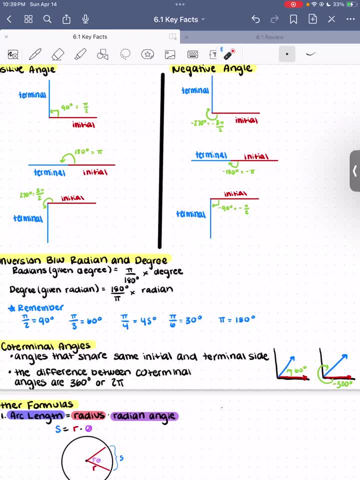 is are two angles. So we're comparing two angles here. Let's say angle A and angle B. So if angle A and angle B are coterminal, that means they share the same initial and terminal side, but they don't have the same angle measure. So 60 degrees if 60 degrees is angle A and 60 degrees. 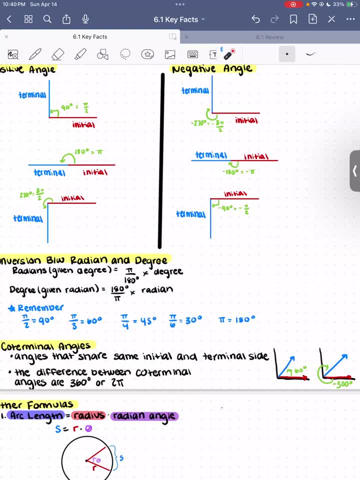 is angle B. that just means they're the same angle. They're not coterminal angles. They're just the same angle. So how do we know if they are coterminal angles? So we know that as if the difference between the two angles are either 360 degrees or 2 pi radians. So 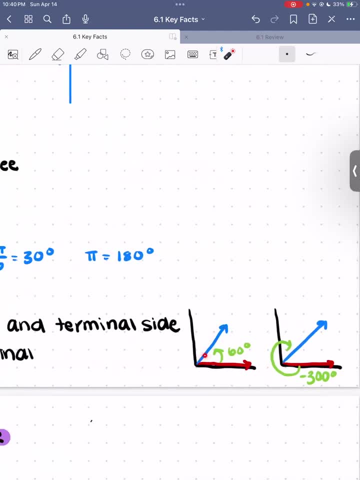 if we look at my little example right here, you can see they have the same terminal side and the same initial side. However, if we were to measure this coterminally- whoa, if we were to measure this counterclockwise, we would have gotten 60 degrees. However, 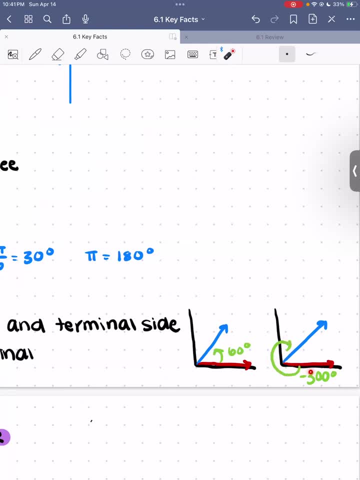 if we were to measure this exact same thing, but clockwise, we would have gotten negative 300 degrees, And since, if you were to do negative 300 minus 60, that's negative 360. And therefore they are 360 degrees apart. 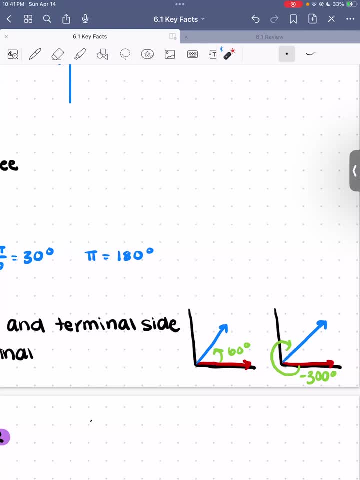 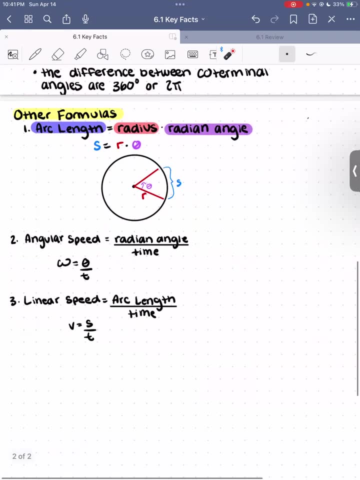 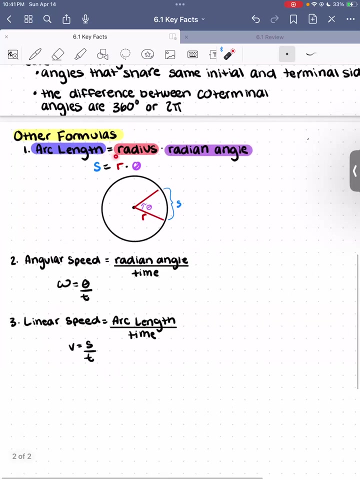 Which means 60 and negative 300 are coterminal angles. Okay, Some other important formulas that we need to know and that'll help you in 6.1, is our arc length, angular speed formulas and linear speed formulas. So for arc length, arc length is equal to our radius times, our 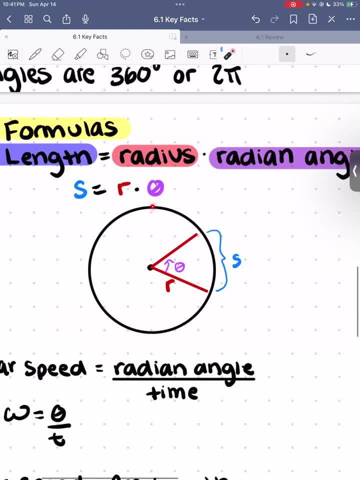 radian angle And the radian, and if we look at this right here, so we have a full circle. If this is the origin right here, our radius is the point from the origin to the outer edge of the circle, always from the point of origin to the edge. It can't. 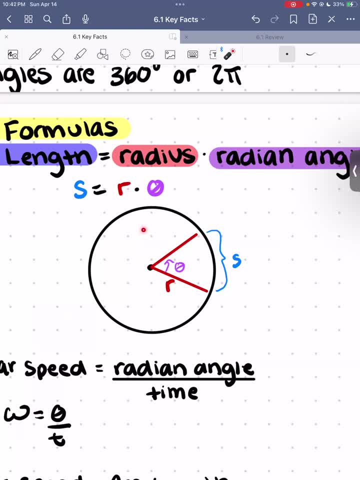 be from anywhere else. So we can't say like, oh, here, from here. No, The radius is always from the center of the circle to the edge. Our radian angle is: if so, technically, this line right here is still our radius. 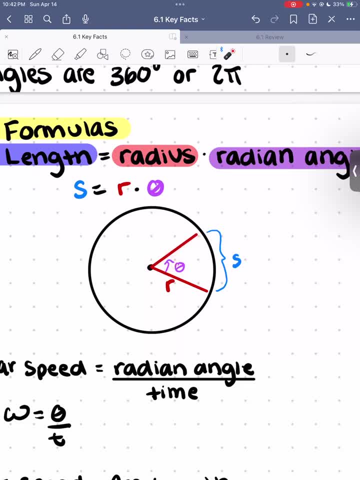 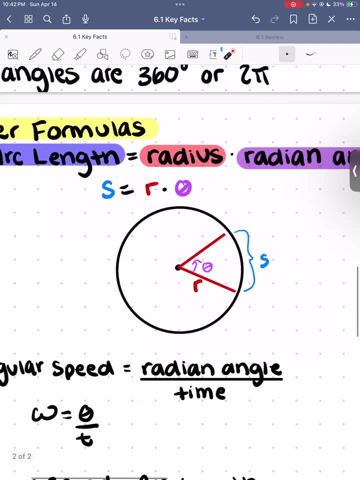 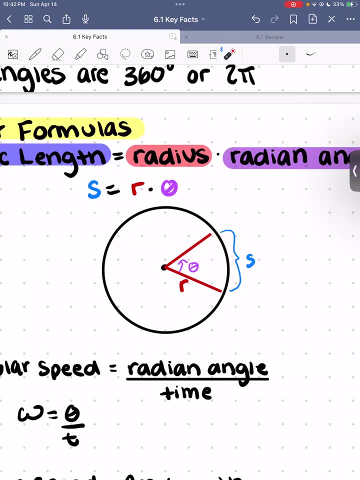 Okay, If we compare the angle between our two slices that we've made, it'll give us our radian angle Usually given but sometimes not, depending on what they want you to find. And then our arc length is the length of the circle between our two points where our radiuses touch the. 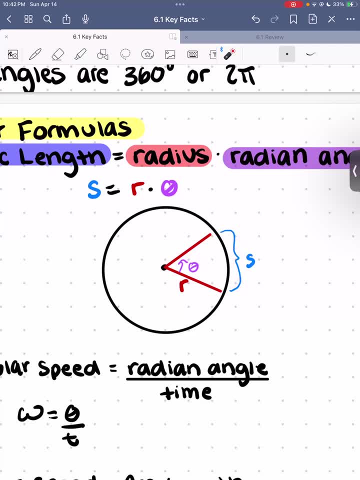 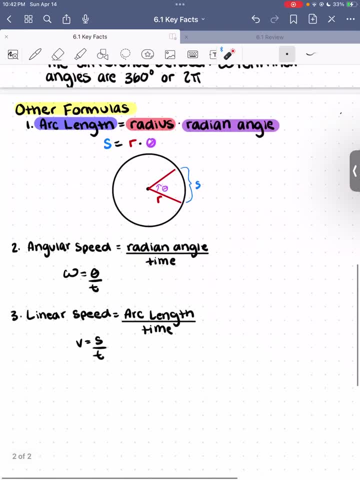 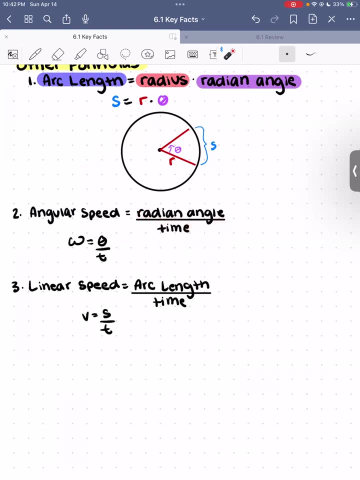 edge of the circle. So if you just take your radius times, your angle, that will give you our arc length. Okay, Now that we have our our radian angle that we just made, then we can see that we have our radian angle over time. Do we see the great red? and the red means we're temperature. 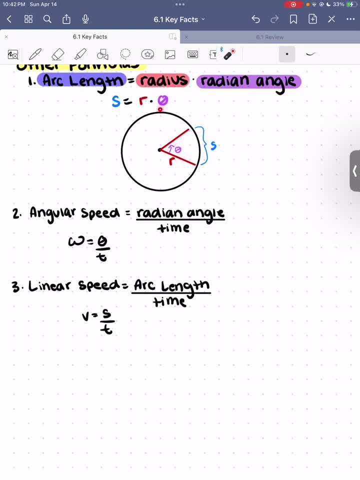 neutral. Okay, So angular speed is our radian angle over time. So remember, our radian angle is just theta. That is what this symbol is. it is theta And it could also be written as: omega is equal to theta over t. Remember this is not W, This is angular speed is shown as: 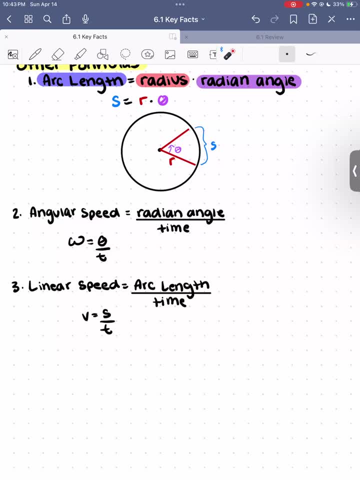 omega, Which is a Greek symbol. look like W, but it is different. But yeah, that's all. angular speed is, And then linear speed is our arc length over time. So remember, our arc length is the measure of the distance between two points on the circle, And so that can be written as: V is equal to S over T.